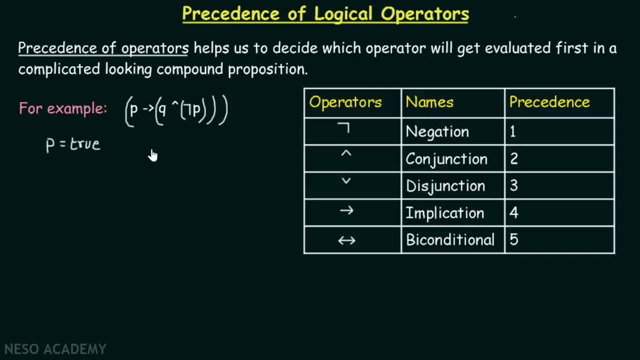 P is true and Q is false, Then what would be the truth value of this compound proposition? Let me write this compound proposition once again: As P is true, therefore not, P becomes false And Q is also false, therefore false and false. 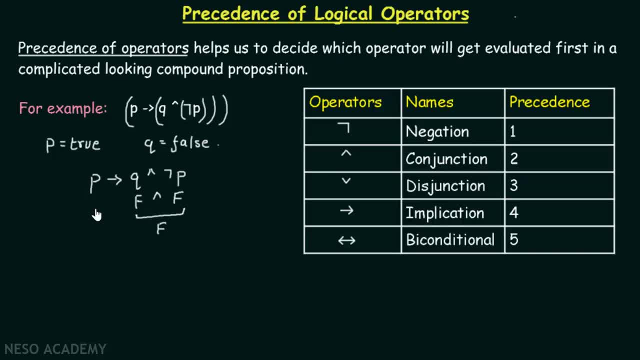 becomes false As P is true and this whole compound proposition is false. therefore, true implies false is finally false. This would be the truth value of this compound proposition. P implies Q and not P If we directly go, without using the precedence table. 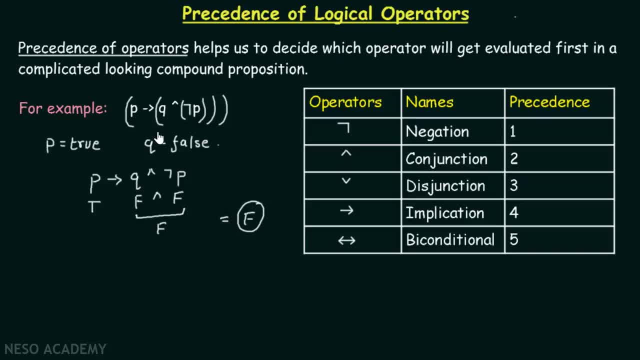 then it may produce different result. Therefore, precedence of operators is very important for us to know. Now let's consider one problem: Construct the truth table for the compound proposition below P implies not Q and not P equivalent not Q. So this is the bi-conditional operator. 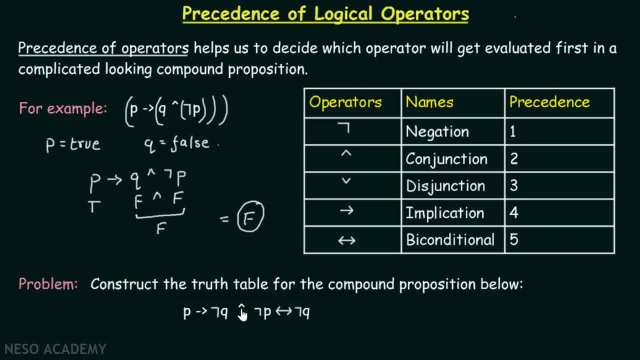 negation operators: conjunction operator and implication operator Right. Of course this is quite complicated looking compound proposition and without knowing the precedence of operators we cannot calculate the truth value of this compound proposition. Here we need to construct the truth table Now. 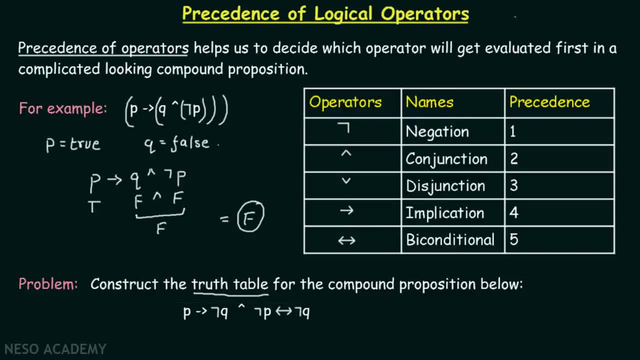 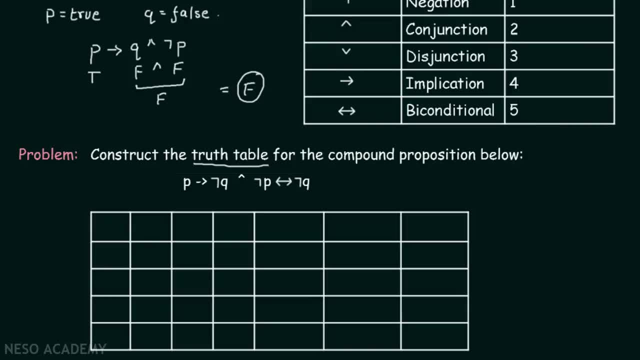 let's construct the truth table. Okay, Let's write all the different combinations of P and Q first. First combination is true-true, then true-false, then false-true and then false-false Right After that, as we need to calculate. 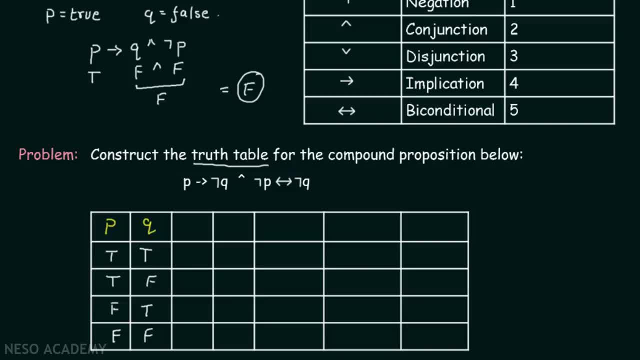 not P and not Q. we have two combinations of not P as well as not Q. As P is true, not P becomes false. Again, P is true. therefore not P becomes false. This one will be true and this one will be true.